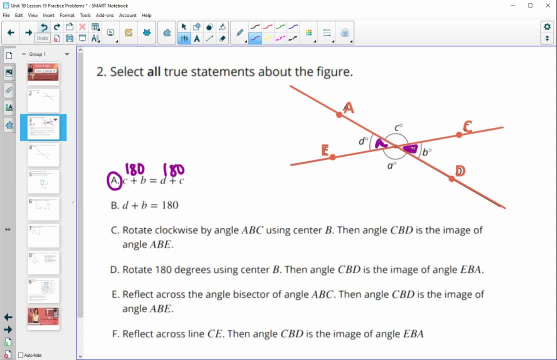 is equal to 180. Those are vertical angles, they're across from each other, so they don't necessarily equal 180, they would equal each other, so D would equal B, but we don't know that they equal 180. Then it wants us to rotate clockwise by angle ABC. so by angle ABC, meaning we're going to 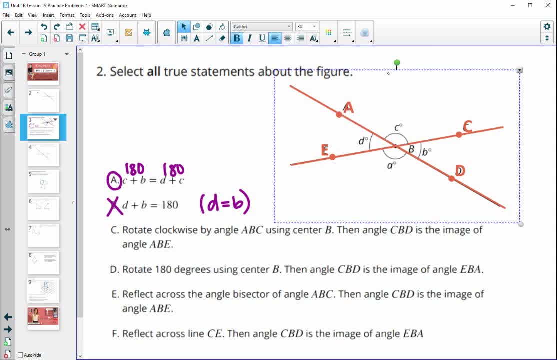 want to rotate this ray down to this one, so let's do that. so rotate by angle ABC. so I rotated this side of the angle over, then angle CBE. so angle CBE, or, sorry, CBD, will be the image of EBA. so did CBD land on EBA? so here's CBD and here's EBA. they are not on top. 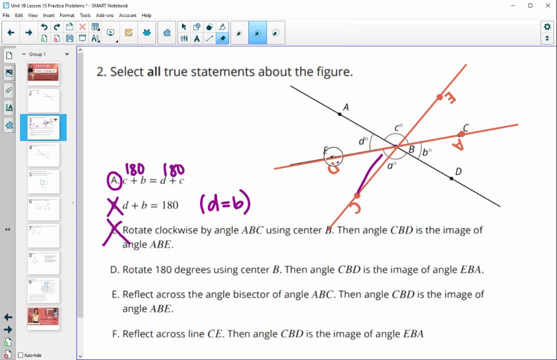 of each other. so they are not images of each other. All right, let me get this out of here, Okay. so then let me put this back. so now it says: rotate 180 degrees, using B as the center. is angle CBD, the image of EBA. so do they land on each other? so now we're going to go 180 degrees. 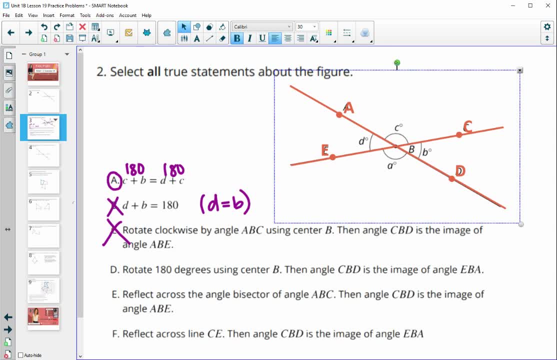 so you're going to see this orange A go all the way over to here. so we're going to rotate 180 degrees. now is angle CBD, so here's CBD, the image of ABE, so the original, so black ABE is right here. 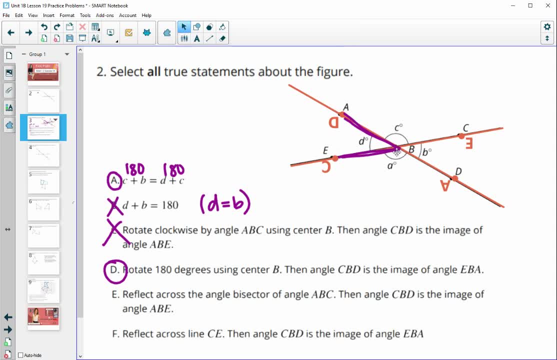 those are on top of each other, so they are images of each other. after that 180 degree rotation, So let me get this reset. All right then. E says to rotate reflect across the angle bisector. So let me get an angle bisector drawn in here. So the angle: 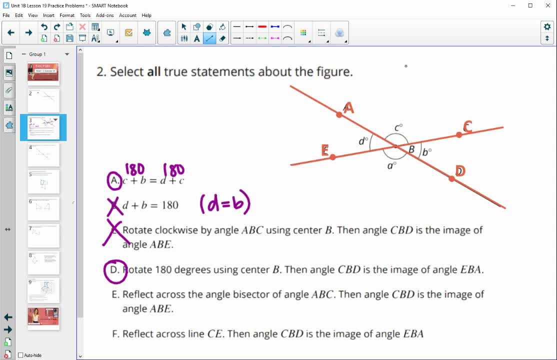 bisector of angle ABC. So here's angle ABC. So the angle bisector would split that in half. And so if we reflect across that, okay, if we reflect across that line, you'll see that these two angles, or that A lands on C, C lands on A, D lands on E, E lands on D, So is angle C, B, D. 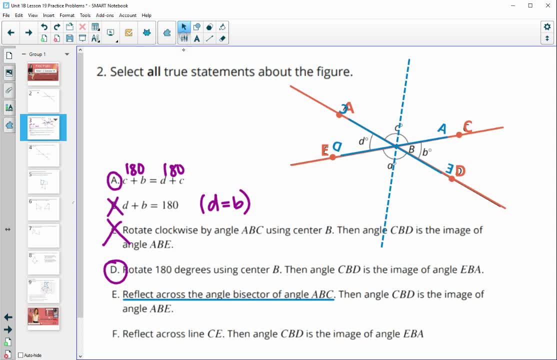 the image of A, B, E, And those two do land on top of each other. So that's a true statement. So let's get rid of this, All right. Then the last one that we want to do is reflect across line CE. So we see CE right here. So if we 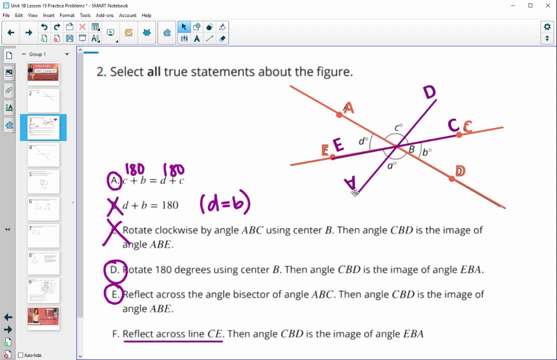 reflect across that line A will flip down to here, E will stay on, the line C will stay on, the line D will flip up. So is C, B, D. does that land on A, B, E? And they do not. So they are not images. 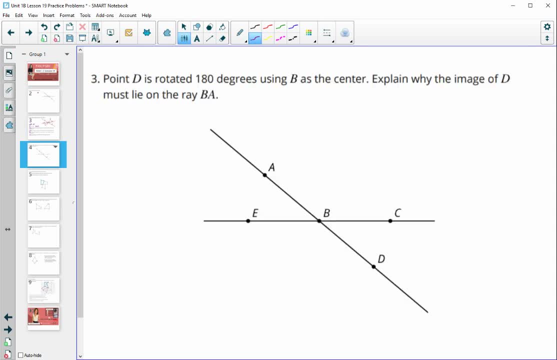 of each other. Number three, point D. So if we rotate this 180 degrees using B as the center, explain why D must land on ray BA. So let's draw ray BA here. So ray BA starts at B and goes this way. So how do we know that D is going to land over here? 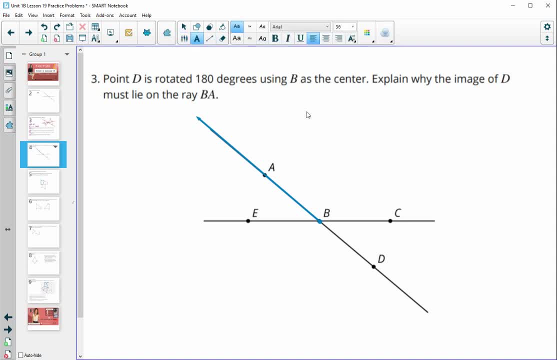 Okay, on that blue ray. So by- let me get this smaller. So we know that, by the definition of a rotation, that when we connect the original to the center of rotation and then to the image, that will make the angle of rotation, 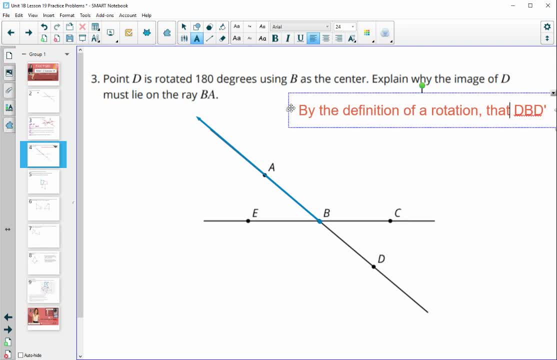 So by definition of rotation we know that D, B, D' is going to land on the center of rotation will be 180 degrees, meaning that D B and D prime will be on a straight line and D prime will need to be on the opposite side of point B after the rotation. So D prime will have 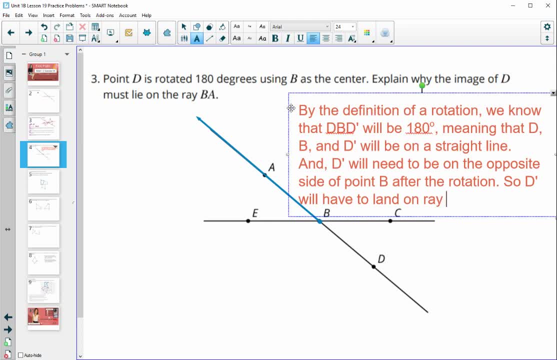 to land on ray BA, since it has to be on the other side of B. So we know through the rotation that it's going to make a straight line and then D is going to rotate and it's going to land on the opposite side of point B. 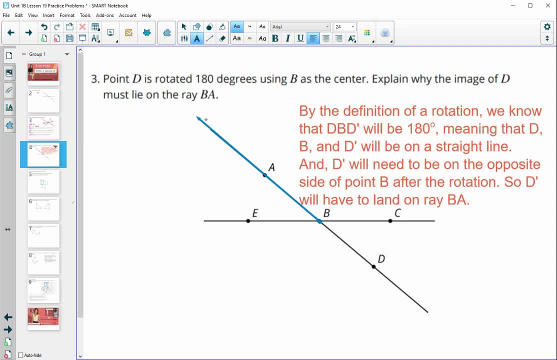 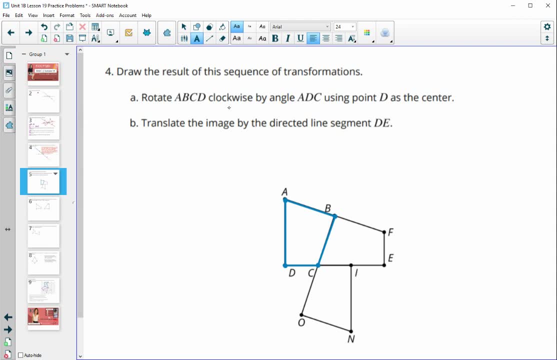 It will be on the opposite side of B, meaning it will have to land on that ray BA. Number four: rotate ABCD, so quadrilateral ABCD, clockwise by angle ADC. Okay, so here's the angle ADC right here. So we're going to have to rotate this down So you'll see this segment land here. 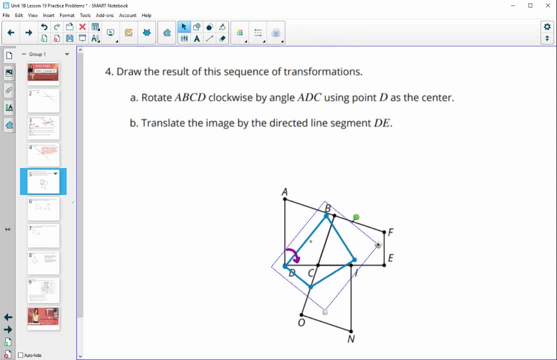 when we rotate and I'll have to keep moving D so that it stays in the same direction. Okay, but we'll rotate until we've rotated that full angle. So we took- and you can see that we moved this side down. Now we're going to translate by directed segment DE, So we're going to take D. 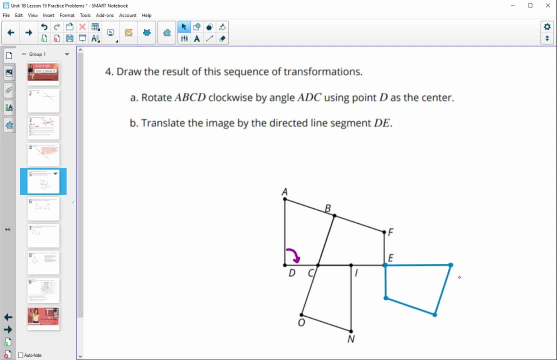 and move it all the way over to E, and then that would be our new image, And then you can just make sure that you label the points. So this one is going to be on the opposite side of point B. So we're going to take D and move it all the way over to E, and then that would be our new image, And then you can just make sure that you label the points. So this one is going to be on the opposite side of point B. 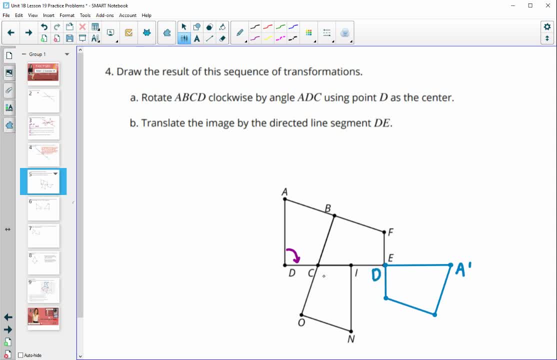 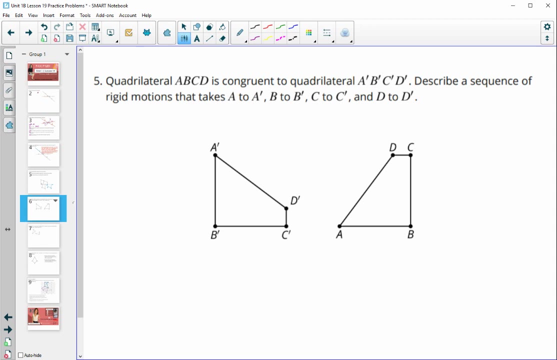 Okay, so this one was our A prime D, B rotated to here, So that was B prime and then that was C prime. Number five quadrilateral ABC is congruent to quadrilateral A prime, B prime, C prime D prime. 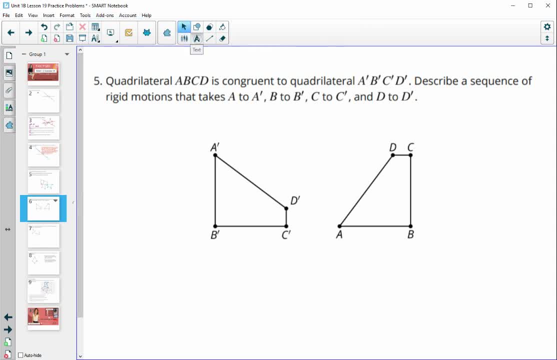 Describe a sequence of rigid motions that will take one to the next. All right, so I'm going to take one to the next. They're not touching each other, so we're going to have to translate. So let's translate A, B, C, D by directed segment, and I like to do alphabetical, So I'm going to move. 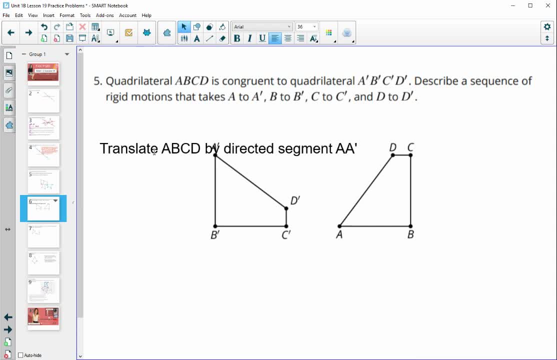 point A to A prime by doing directed segment A, A prime. So this will get A to land on A prime. So once we've done that, so once we've gotten A to A prime, and let's see, I can draw this. 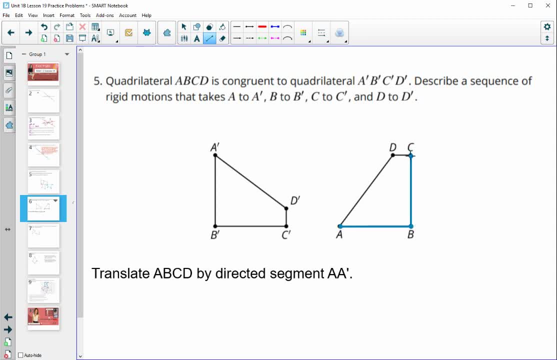 So that we can see this happening. Okay, so now we've got A to land on A prime, Now we're going to want to rotate back, And so this is B. So if we just rotate B down to B prime, then everything will kind. 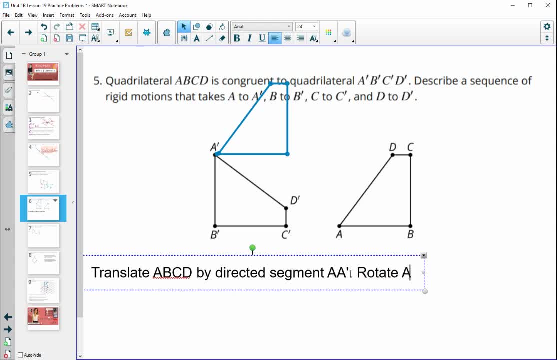 of land in place. So then we will rotate A, B, C, G and D by directed segment. So this is B And so once you're donesn, soaping this, so we're just going to want to rotate those. 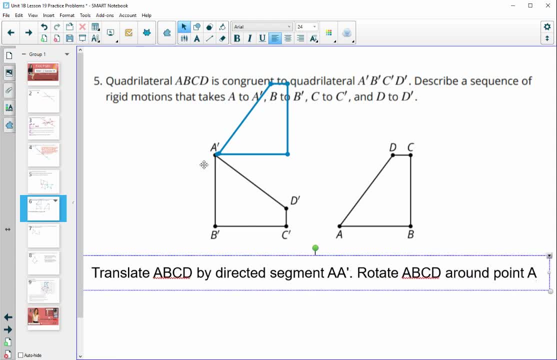 B down to B prime. then everything will kind of land in place. So then we will rotate A, B, C, D and do rated segment A- B prime around point A, the point we just got touching. okay, so the ones that are touching around point. 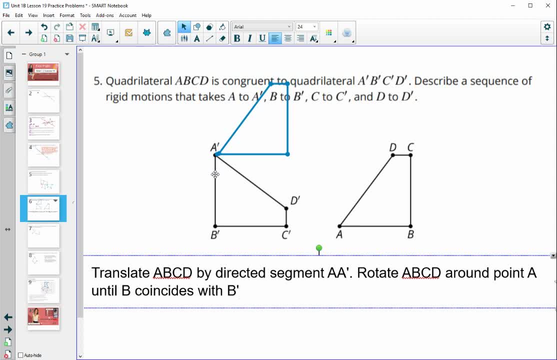 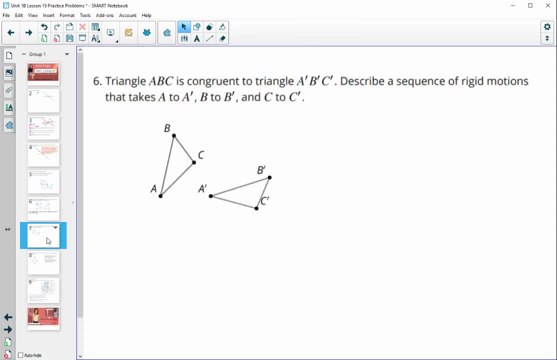 A until B coincides with B prime, That will force then the others to fall in place. Number six: triangle ABC is congruent to A prime, B prime, C prime Again, describe a sequence of motions that will take them to each other. So let's start with a translation, since they're 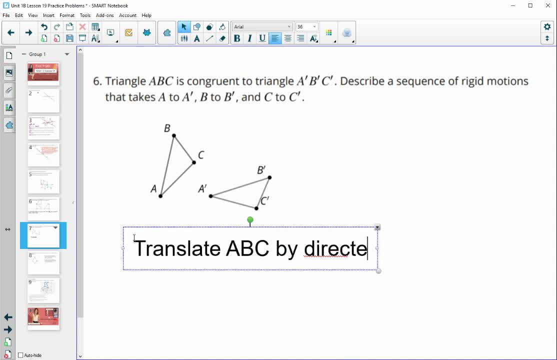 not touching. So translate ABC by directed segment: AA, prime. So now, once we get that, we can see that these points are in the same order. So when we rotate, you know, C to C prime or B to B prime, the rest will fall. So then we can just say: rotate around. well, let's say rotate. 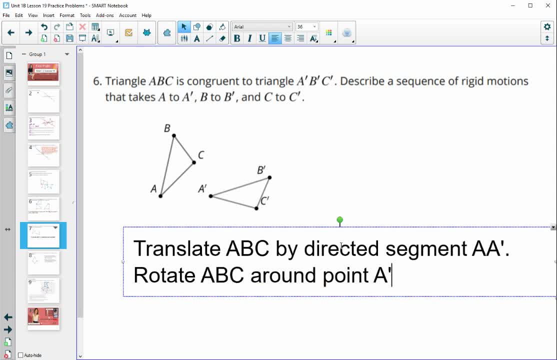 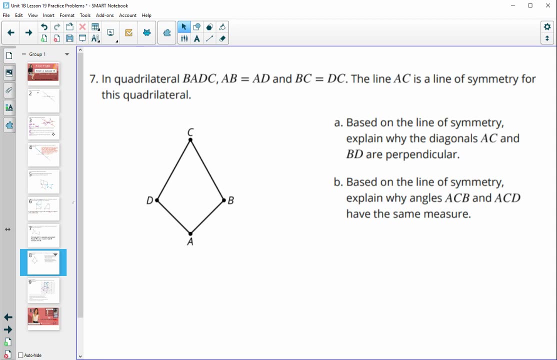 ABC Around point A prime until B coincides with B prime, or you could do C to C prime, whatever you prefer. Number seven: quadrilateral: in quadrilateral, BADC, AB is congruent to AD and BC is congruent to DC Line. AC is a line of symmetry. 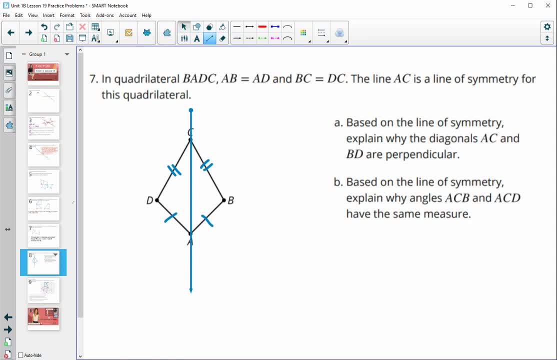 For the quadrilateral. so, based on this line of symmetry, explain why the diagonals are perpendicular. So let's get that written out here, All right. so since we can see that, let me move this. So we can see that A is equidistant from B and D and so is C. So C is equidistant from B and D. 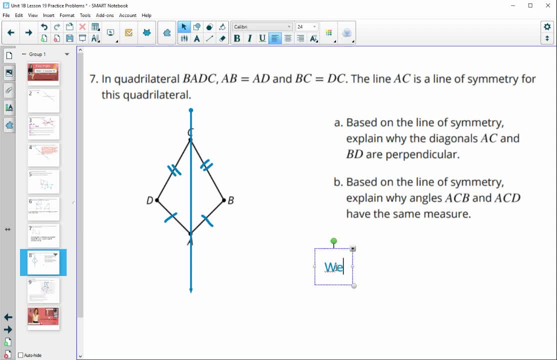 That means that A and C are on the perpendicular bisector. So we can see that A and C are both equidistant from points B and D. Therefore they are on the perpendicular bisector of B, B, D, meaning B, D and A, C are perpendicular. 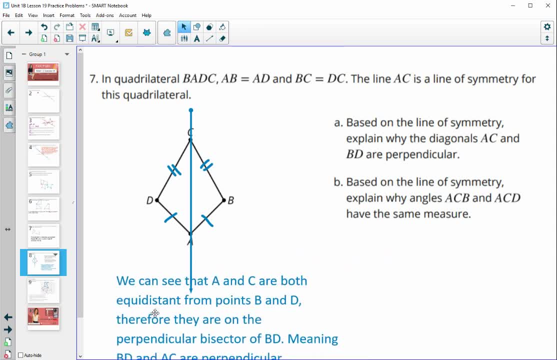 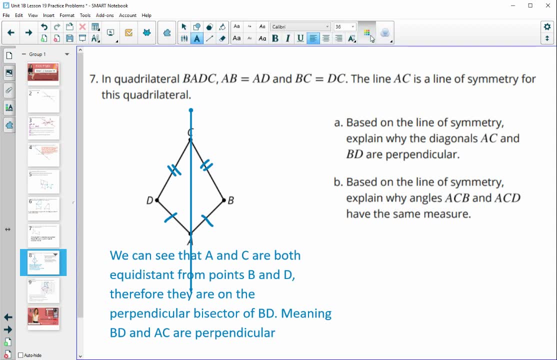 Okay, so that's the answer for part A. Then B says: based on the line of symmetry, explain why the angles have the same measure. So let me change color for this answer. Okay, so for this one, because after the reflection, A and C will stay in place, since they're on the line of reflection. 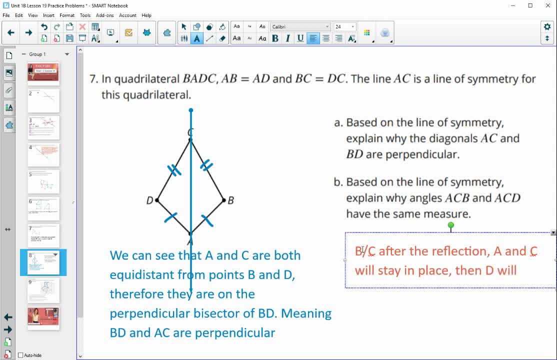 Then D will reflect onto point B. Since um B and B are the same distance away from A, that will mean that A, D, C and A, B, C are equal. So that just means so. since D is the same distance away from A and B, that means D is just going to land right on B. 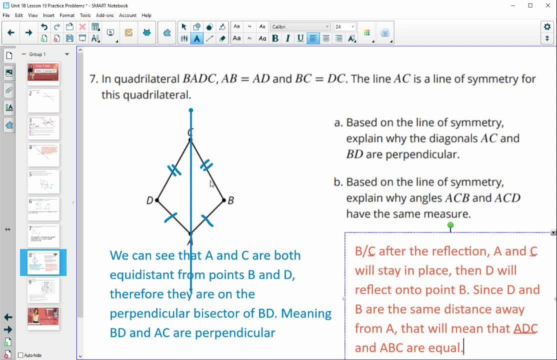 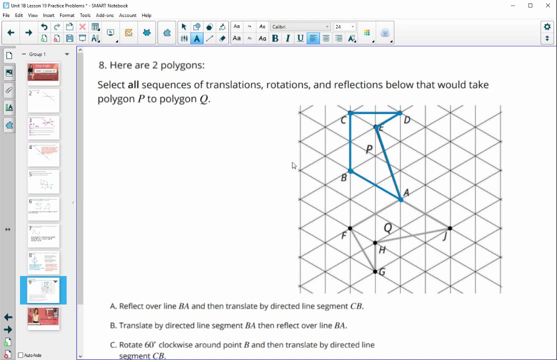 And same thing over here. these two are the same length, So this will fall. D will fall right on B and everything will fall in line since they're congruent. So those two angles have to be the same size, All right. number eight says that we can see a sequence of translations, rotations, or, sorry, select all sequences of translations, rotations and reflections. that would take P to Q. 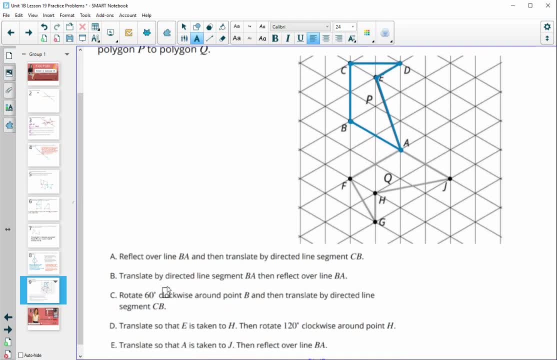 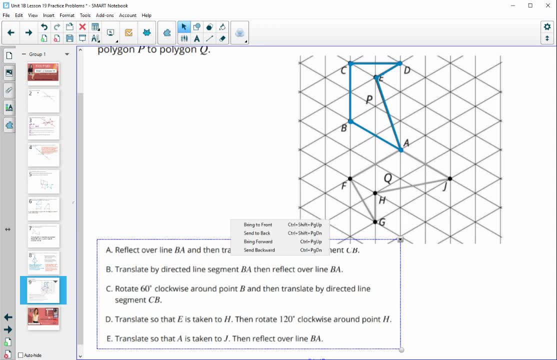 So I've got all of the sequences down here, So let's take a look. So if we were going, and let me pull this up. So if we were going, and let me pull this up. So if we were going, and let me pull this to the front so that it doesn't keep slipping behind there. 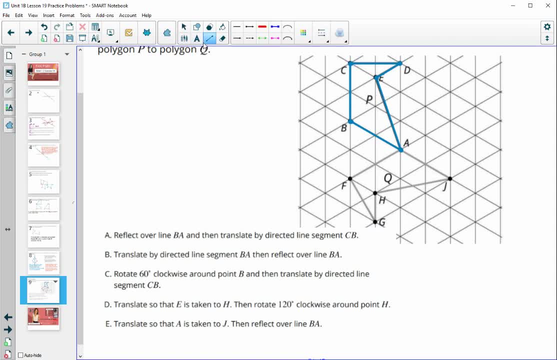 All right. so if we were going to reflect this shape over line B A, we would end up here. Then it says to translate by segment CB. So that's just kind of straight down two triangles. So if we went straight down two triangles here, 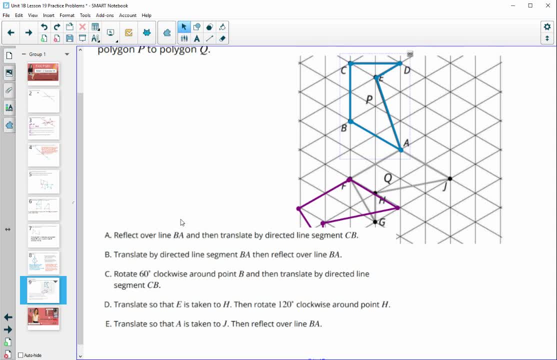 A, it would not land right on top of Q, So A is incorrect. Sorry, So we'll get rid of this. All right. Then B says: translate by directed segment: BA. So we're going to take B, move it down to A. 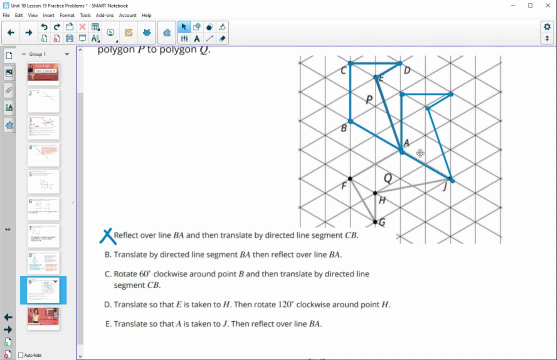 and that's going to just move this shape here. Then reflect overing BA. So if we reflect overing BA, that is going to reflect this whole figure on together on to Q, So that one is going to be good Whoops, All right. Next we're going to want to rotate.